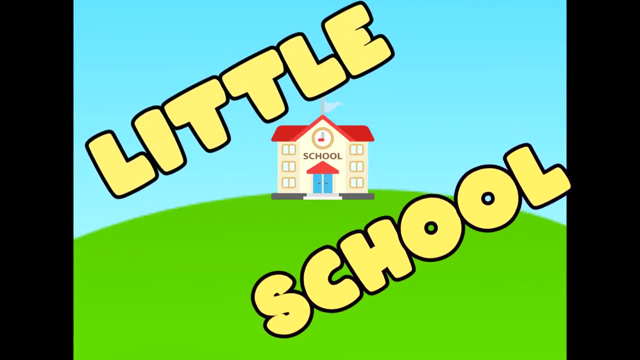 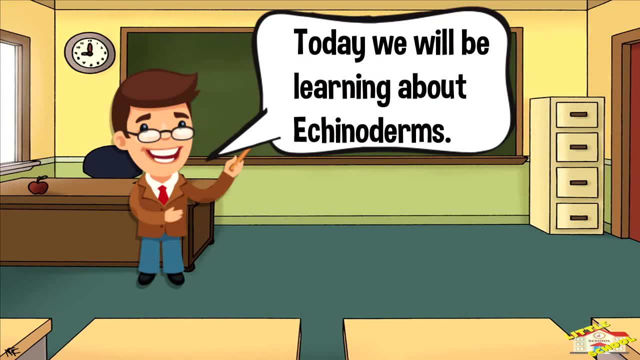 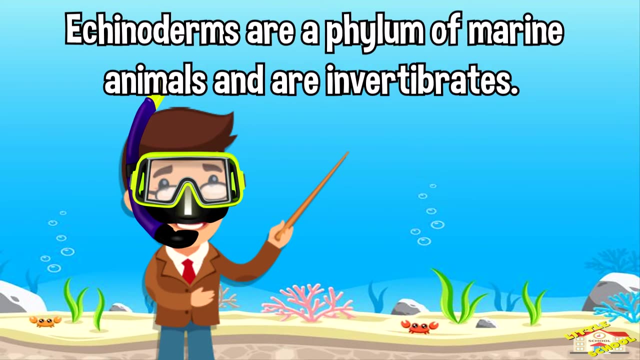 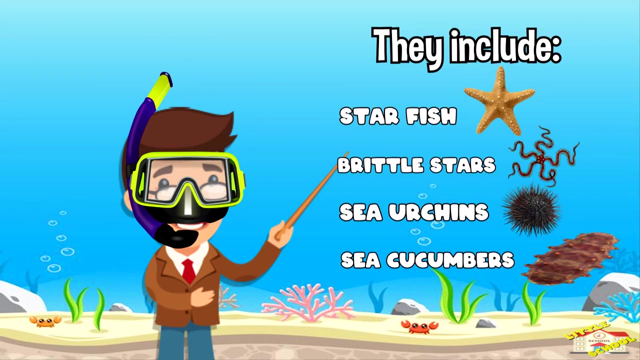 Hey kids, Today we'll be learning about echinoderms. Are you ready? Let's begin. Echinoderms are a phylum of marine animals and are invertebrates. They include starfish, brittle stars, sea urchins, sea cucumbers and their relatives. 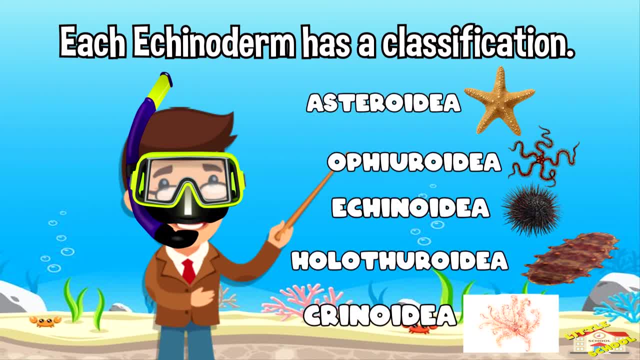 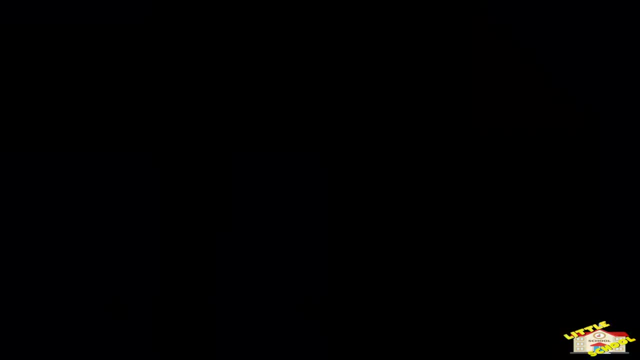 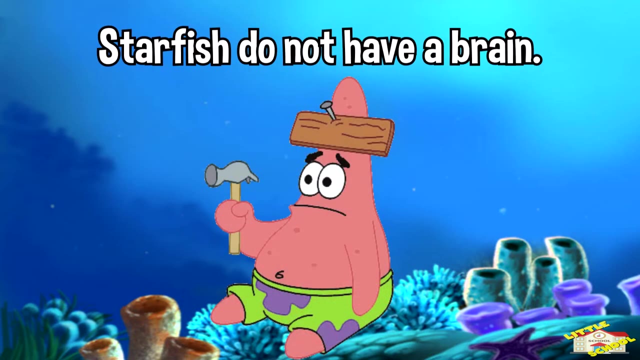 Each echinoderm has a classification: Asteroidea, Hopiroidea, Echinoidea, Holothuroidea and Crinoidea. These are the sea lilies and feather stars. Let's start with the starfish. Starfish do not have a brain. 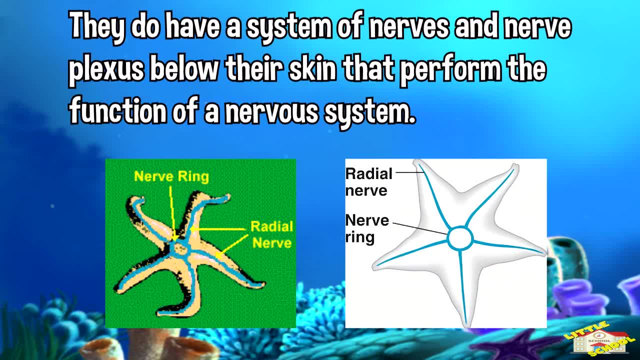 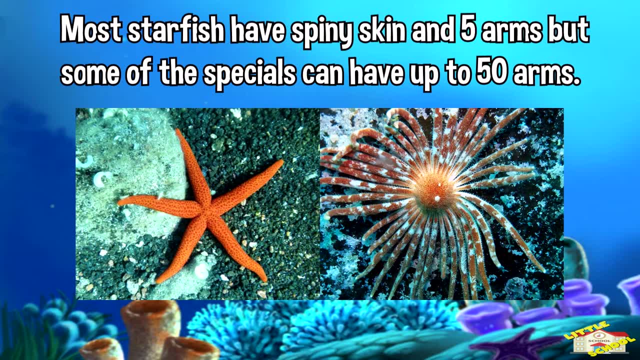 They do have a system. They have a system of nerves and nerve plexus below their skin that perform the function of a nervous system. Most starfish have spiny skin and five arms, but some of the specials can have up to 50 arms. 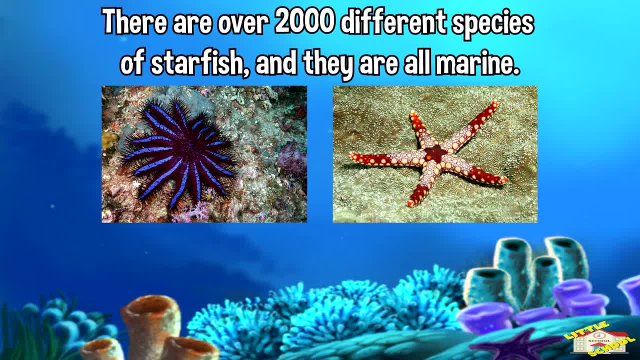 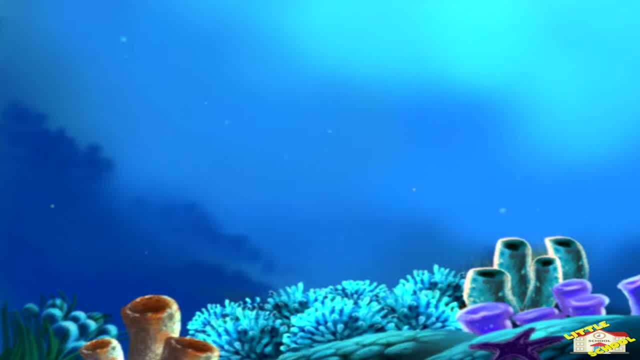 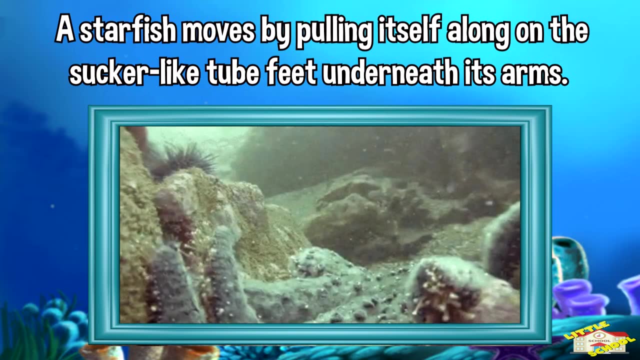 There are over 2,000 different species of starfish and they are all marine. They cannot be found in freshwater lakes or rivers. A starfish moves by pulling itself along on the sucker-like tube. Its arms get stuck in a net and pierce the inside of its body. 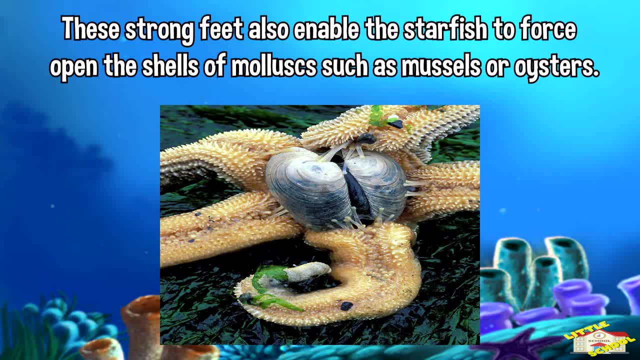 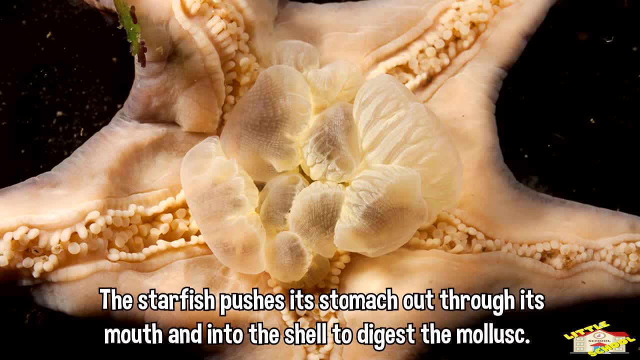 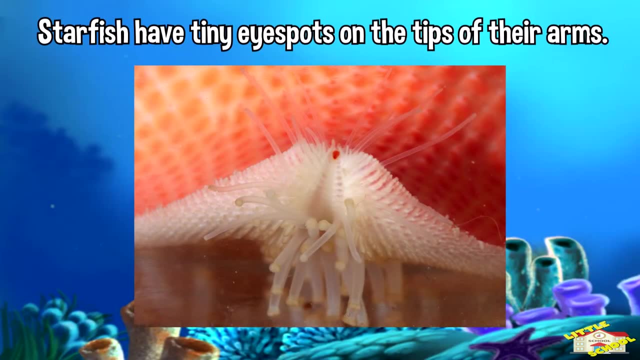 The starfish's trunks also have many fins. They have long legs and wide feet. They have three arms, two feet and three feet underneath its arms. These strong feet also enable the starfish to force open the shells of mollusks such as mussels or oysters. 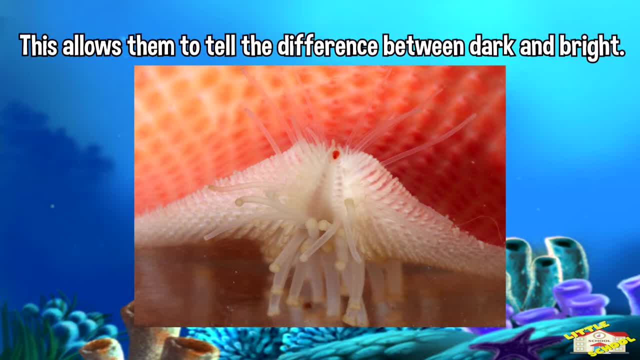 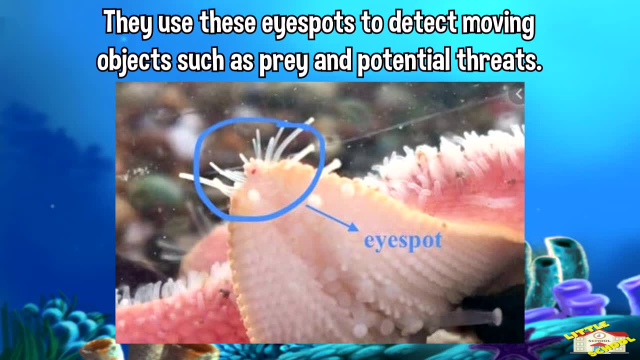 The starfish pushes its stomach out through its mouth and into the shell to digest the mollusk, them to tell the difference between dark and bright. They use these eye spots to detect moving objects such as prey and potential threats. They have an incredible ability to. 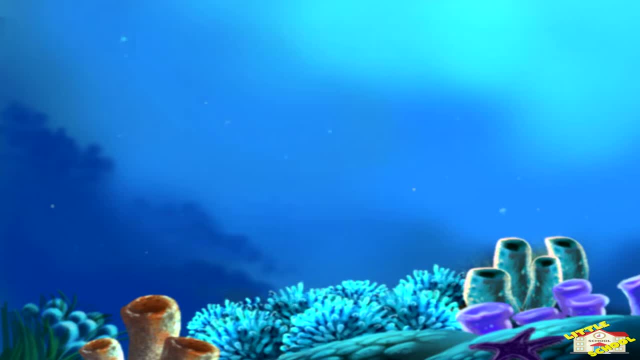 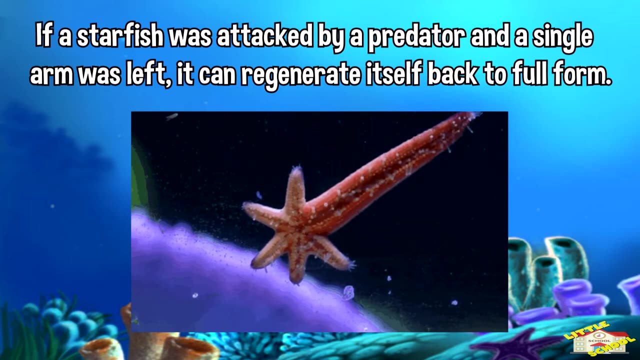 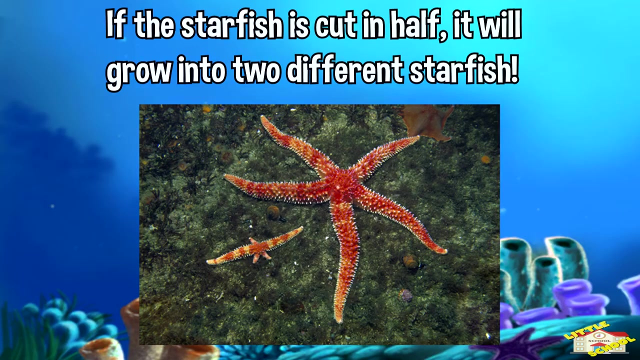 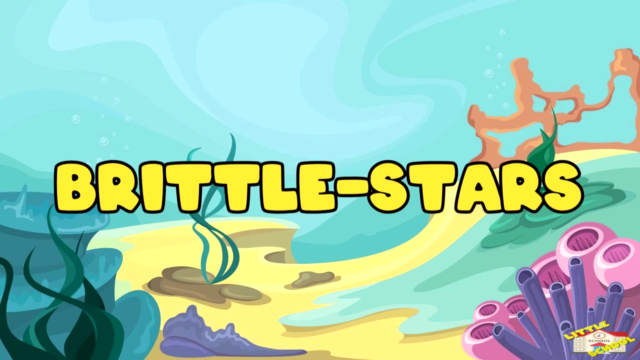 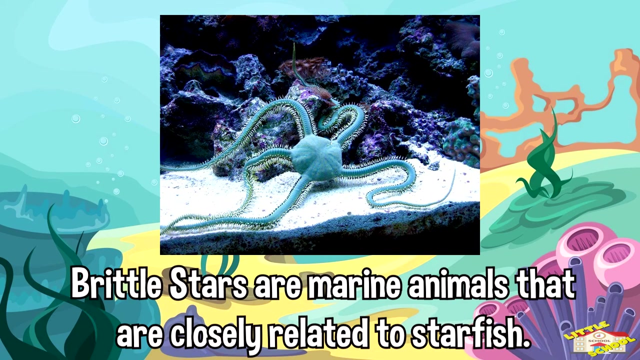 regenerate. If a starfish was attacked by a predator and a single arm was left, it can regenerate itself back to full form. If the starfish is cut in half, it will grow into two different starfish. Next would be Brittle Stars. Brittle stars are marine animals that are closely related. 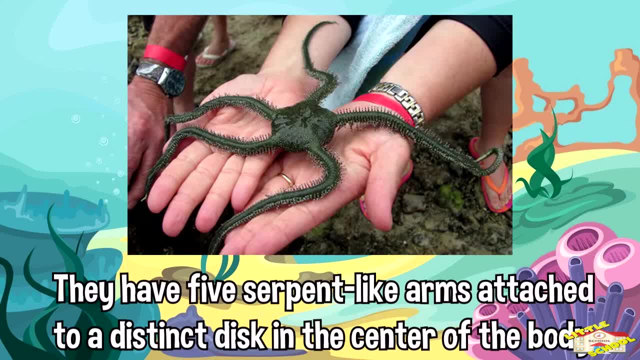 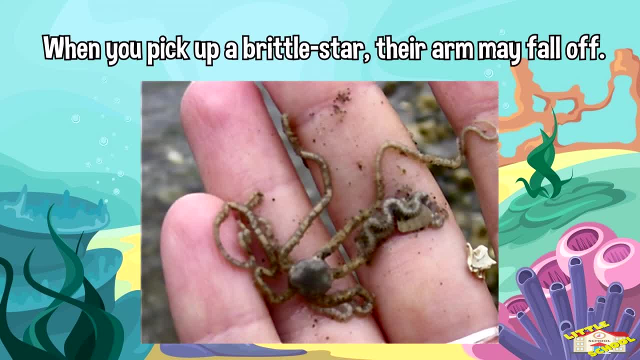 to starfish. They have five serpent-like arms attached to a distinct disc in the center of the body. When you pick up a brittle star, their arm is shaped like a star. They are also known as the starfish. They are also known as the. starfish. They have five serpent-like arms attached to a distinct disc in the center of the body. When you pick up a brittle star, their arm is shaped like a star. They are also known as the starfish. They have five serpent-like arms attached to a distinct disc. 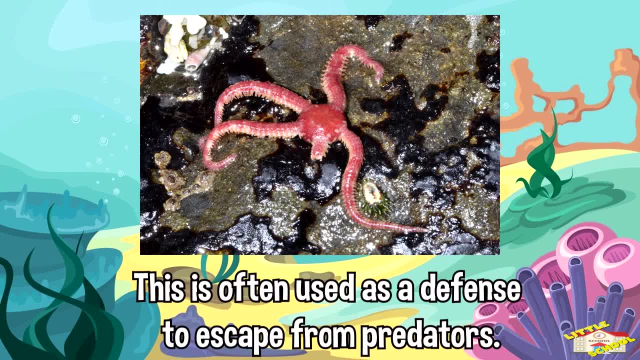 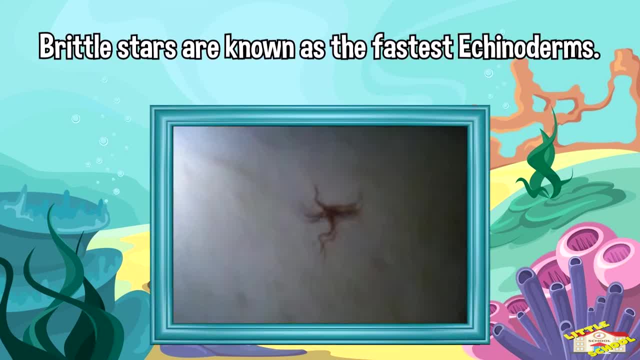 in the center of the body. When you pick up a brittle star, their arm is shaped like a star. They are also known as the starfish. They are also known as the starfish. This is often used as a defense to escape from predators. Brittle stars are known as. 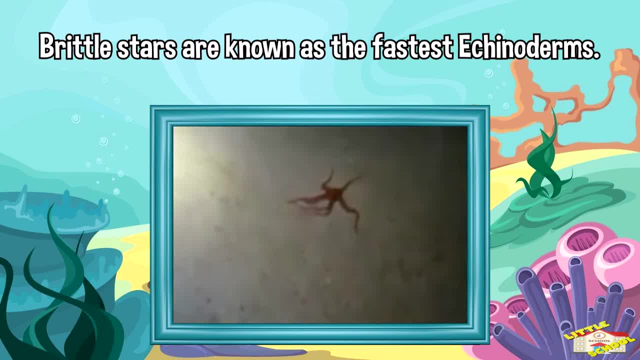 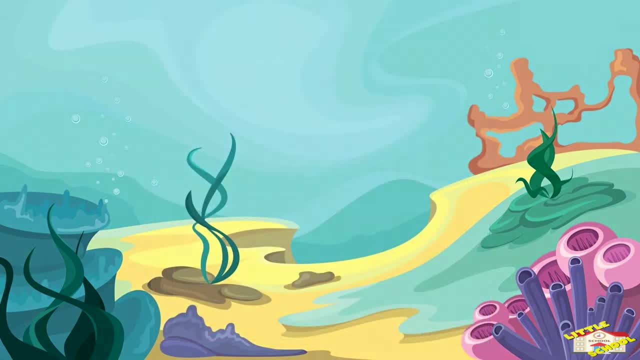 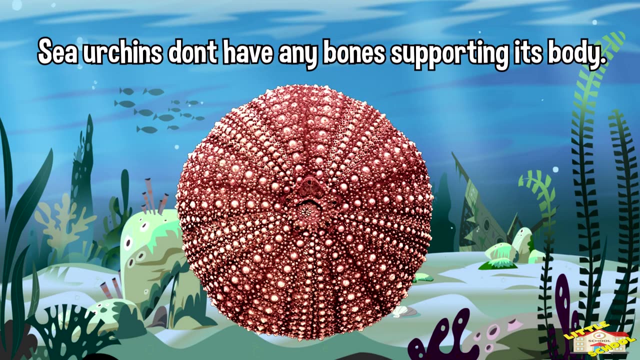 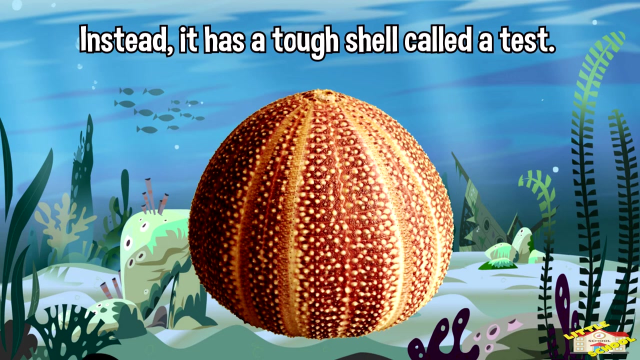 the fastest echinoderms. They use their highly flexible arms to move across the ocean floor. The Sea Urchin- Sea urchins don't have many eyes. They are known to have bones supporting its body. Instead, it has a tough shell called a test. Its main. 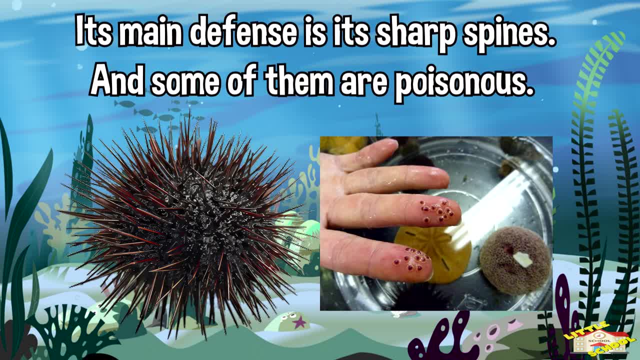 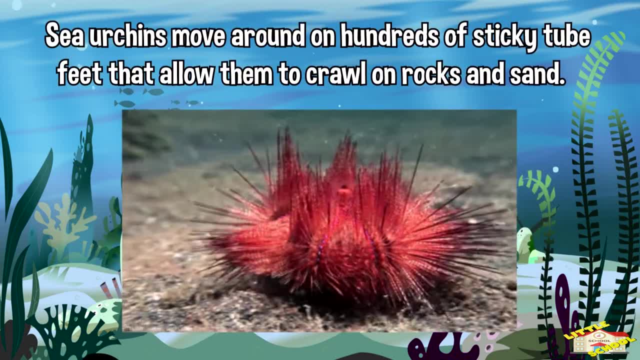 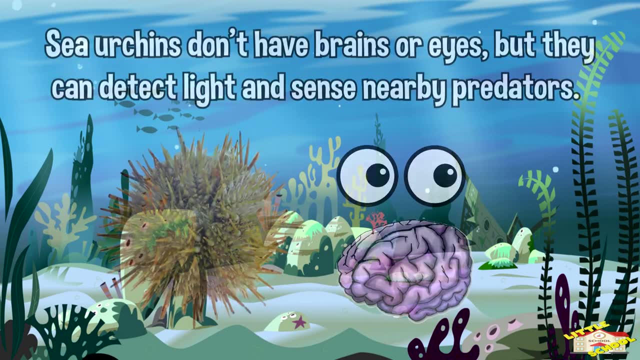 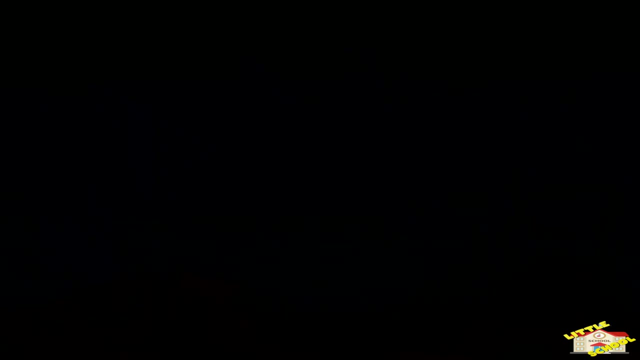 defense is its sharp spines, and some of them are poisonous. Sea urchins move around on hundreds of sticky tube feet that allow them to crawl on rocks and sand. Sea urchins don't have brains or eyes, but they can detect light and sense nearby predators. 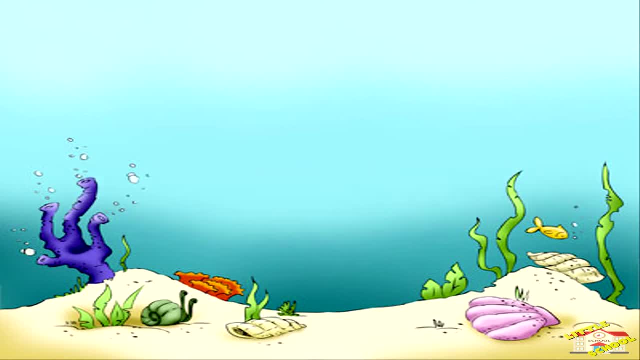 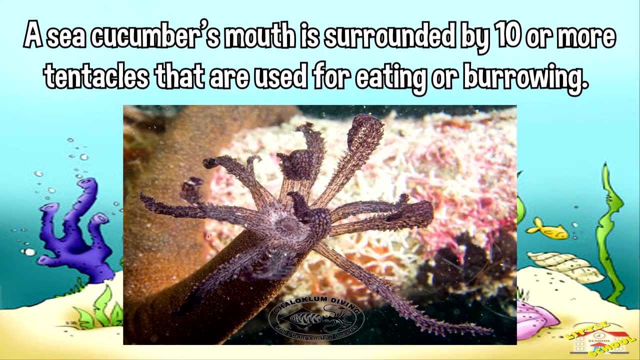 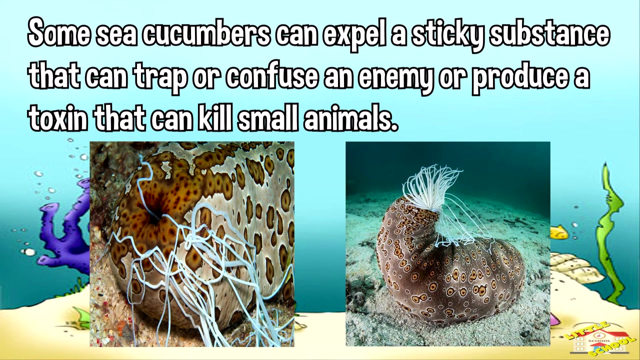 The Sea Cucumber. The sea cucumber's mouth is surrounded by ten or more tentacles that are used for eating or burrowing. Some expel a sticky substance that can trap or confuse an enemy. Others produce a toxin that can kill small animals. The anal opening is used.